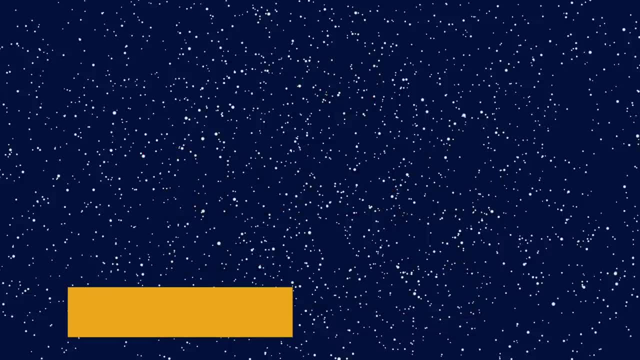 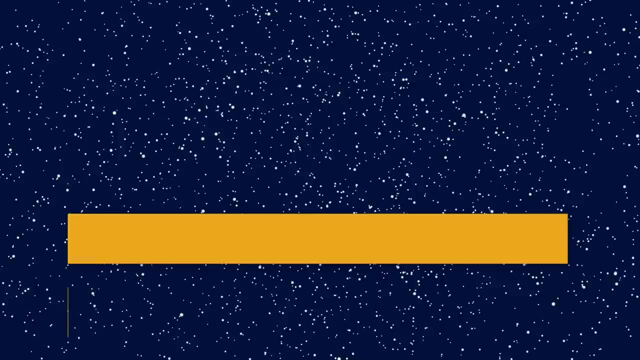 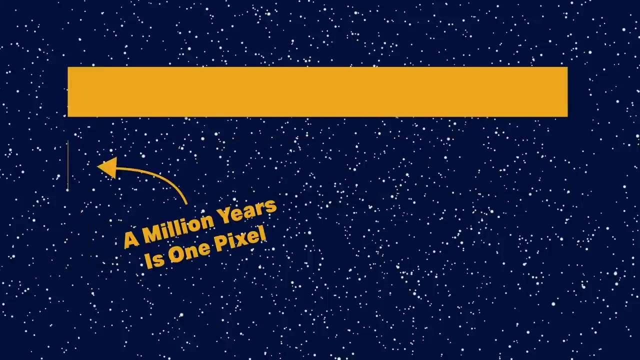 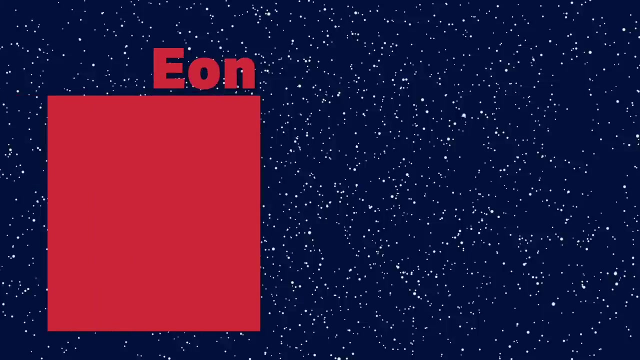 4.6 billion years is a long time. Let's say this represents 100 years, or about a human lifespan. That human lifespan is only one pixel if we zoom out to 100,000 years. We'd then need 10 of those to get to a million years. To get to a billion years, we'd have to add that up a thousand times. That's a really long time. There are so many Earth birthdays that we have to arrange them into phases. These phases are sometimes called eons. 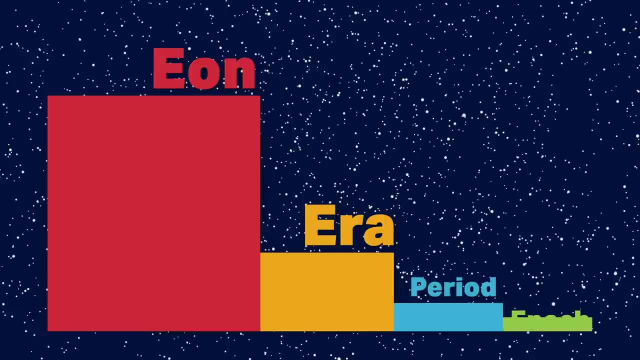 The eons are broken up into eras, which are broken up into periods and epochs. Geologists are apparently fond of words that start with the letter E. 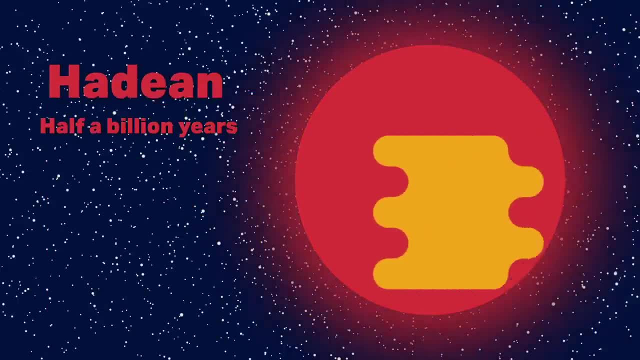 The first eon is called the Hadean. It's about half a billion years when the Earth is just a hot ball of rock, and the moon is just a ball of rock. The moon is forming. What's up, moon? 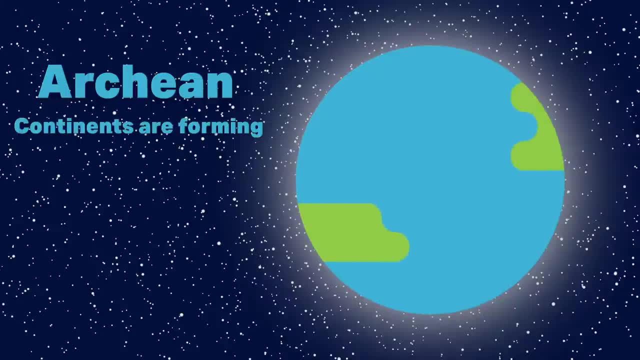 Next is the Archean. Everything has chilled out a bit by now, and the continents are forming. This takes a really long time, almost 1.5 billion years, and life is starting to form in the oceans. 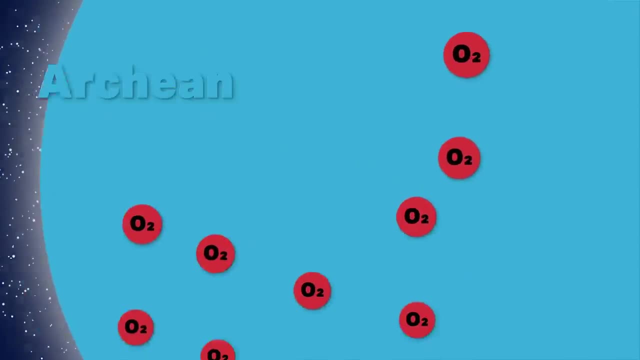 As the Archean is ending, that new life starts to fart out oxygen into the atmosphere. 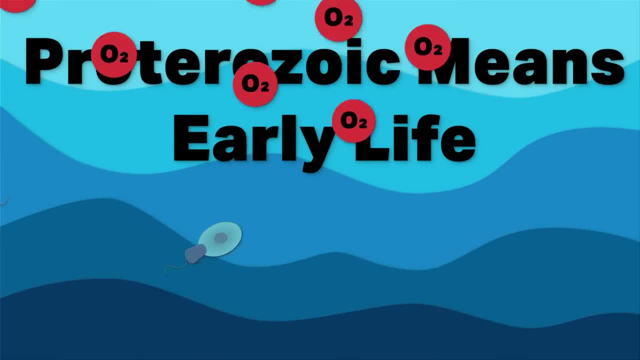 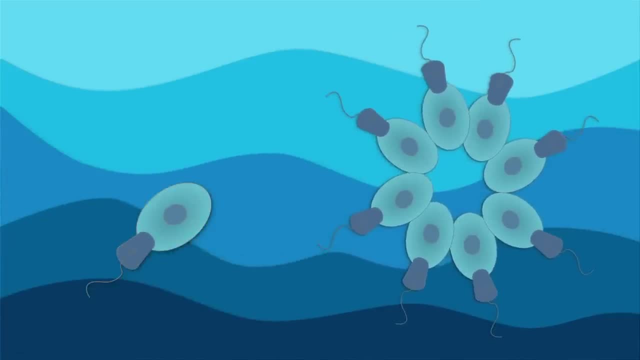 After that is the Proterozoic, which means early life. But it really means very small life. During the Proterozoic, we get the first complex cells, and the first things that are made up of more than one cell. The Proterozoic is also very small. The Proterozoic is very long, about 2 billion years. 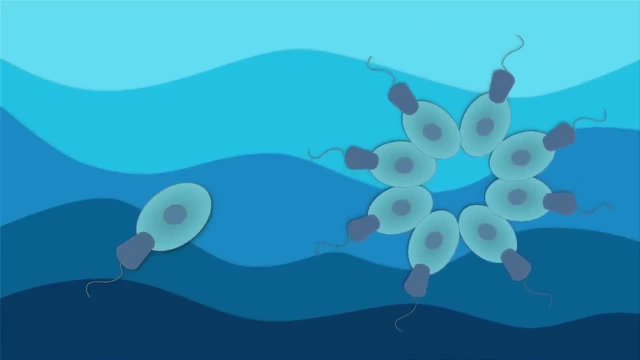 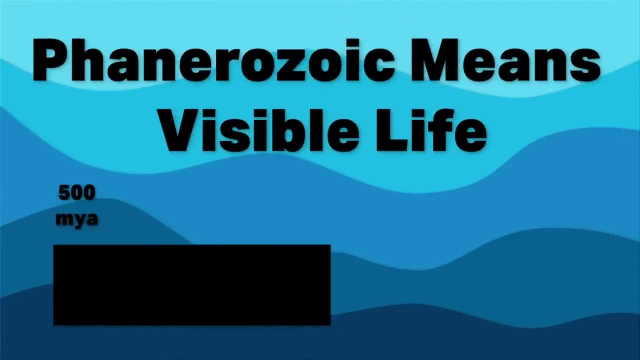 As the Proterozoic is ending, we get the first plants and the first animals. The final eon is called the Phanerozoic, which means visible life. It started about 500 million years ago with an explosion of new and crazy-looking living things, and continues to this day. 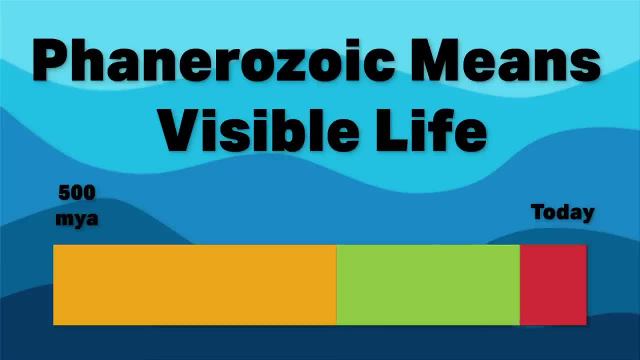 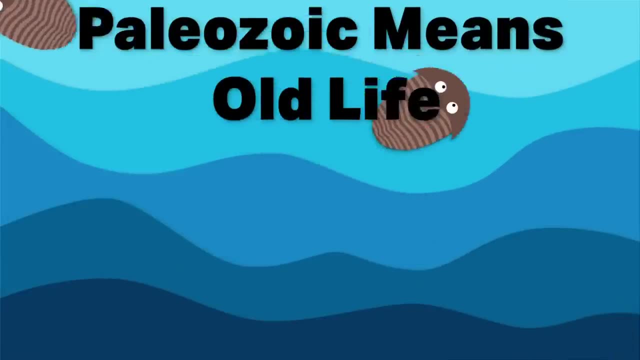 It's divided into three eras. The first era is called the Paleozoic, which means old life. But what it really means is squiggly life, or weird, wormy life. It also means creepy-crawly life. 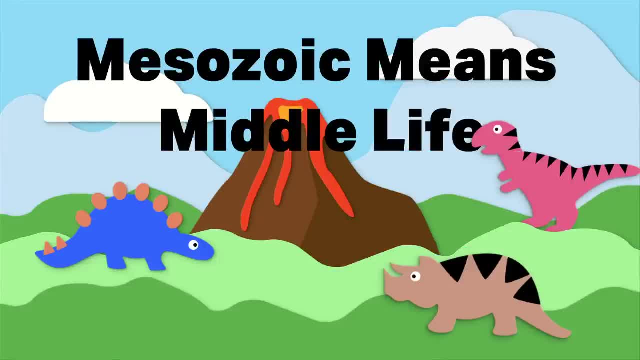 Mesozoic means middle age. But it really means dino-life, or life that goes roar. The Mesozoic ended with a giant asteroid that killed almost everything that went roar. The third era, the Cenozoic, means new life. But it really means furry life, and flappy flying life.